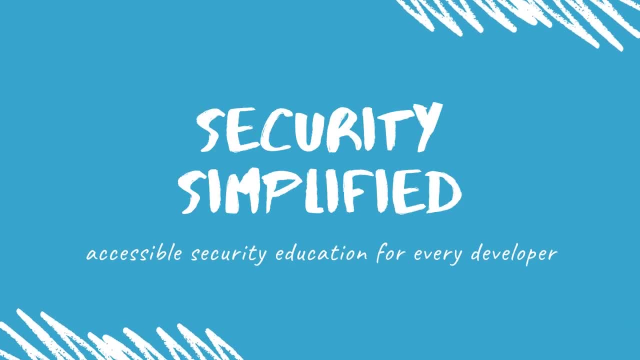 Welcome back to Security. Simplified. Performing a source code review is one of the best ways to find security issues and vulnerabilities in an application. But how exactly do you do it? So today, let's establish a basic framework that you can use to analyze your code, to find 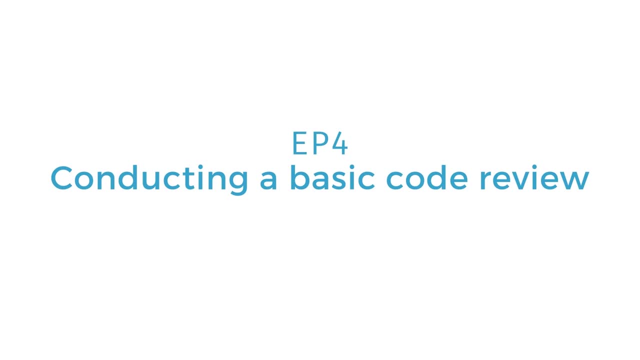 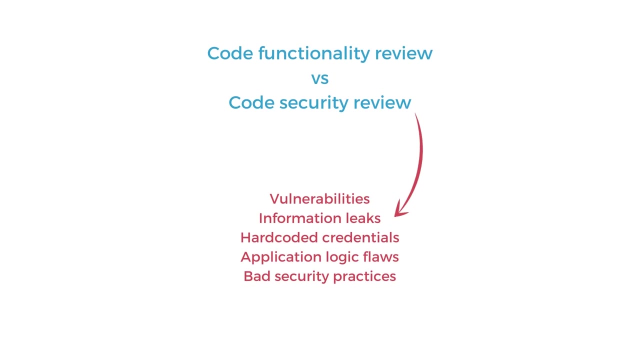 security vulnerabilities. You're probably already familiar with the code functionality review, where you are verifying if a functionality in your application behaves as it should And, in contrast to that, in a security code review, we are specifically looking for pieces of code that will lead to security vulnerabilities. These could be common vulnerabilities, like 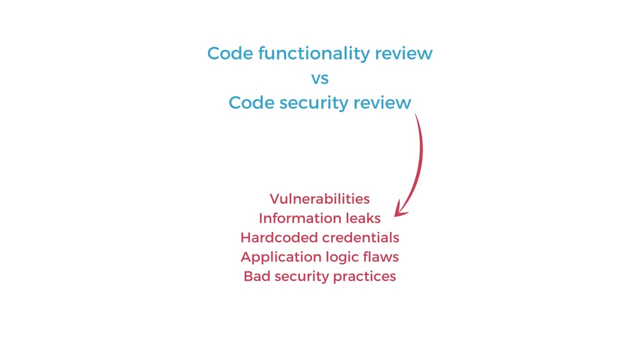 cross-site scripting, SQL injection or bugs like Sensitive Information League or hard-coded credentials or application logic issues that can have a negative impact on your application or its users or your business. So before we get started, let's start by talking about security vulnerabilities. 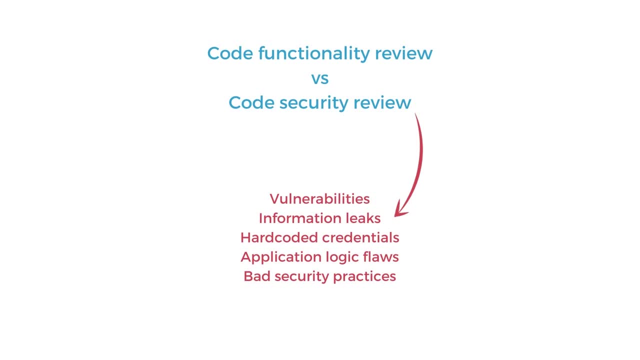 Let's first discuss a few code analysis concepts that you need to understand in order to do this. well, In the code analysis world, a source refers to the code that allows a vulnerability to happen, whereas a sink refers to where the vulnerability actually happens. 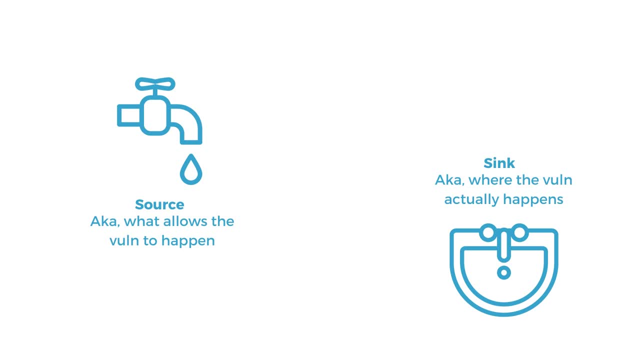 Take command injection vulnerabilities, for example. A source in this case could be a function that takes in user input, whereas a sink would be functions that execute system commands. If untrusted user input can get from the source to the sink without proper sanitization or validation, 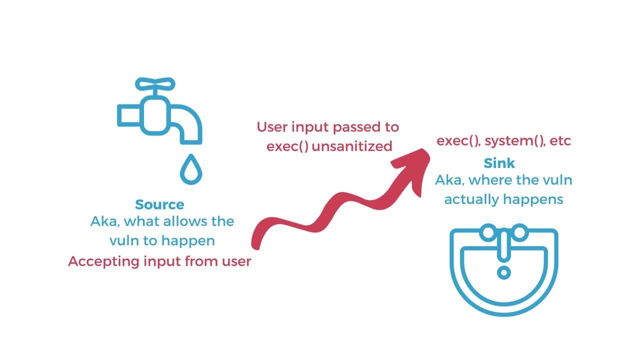 there is a command injection vulnerability there, And a lot of common vulnerabilities can be identified by tracking this data flow from appropriate sources to their corresponding sinks. So first of all, before you actually start reviewing your code for vulnerabilities, start by learning what the most common vulnerabilities are for your application. 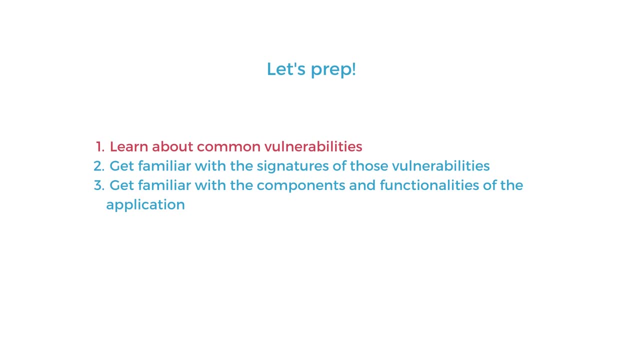 For instance, if you are reviewing an application with many different users, then information leak issues are pretty common, And if your application lets users interact with a database, then SQL injection issues might be something good to look out for. So knowing what the major vulnerabilities are for your application type and getting 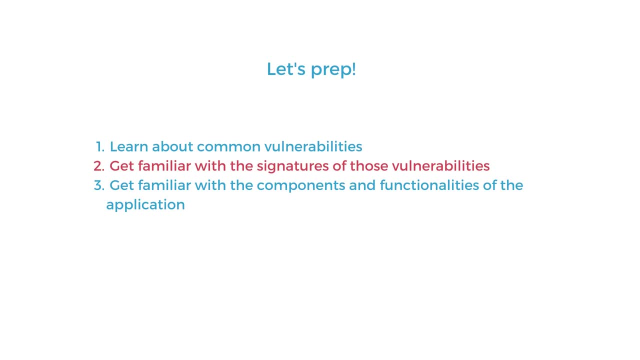 familiar with the indicators and signatures of those vulnerabilities will help you identify similar vulnerabilities. So let's get started. For instance, the signature of an XXE vulnerability or an XML external entity vulnerability is applications passing user-supplied XML to a parser without disabling DTDs or external entities. 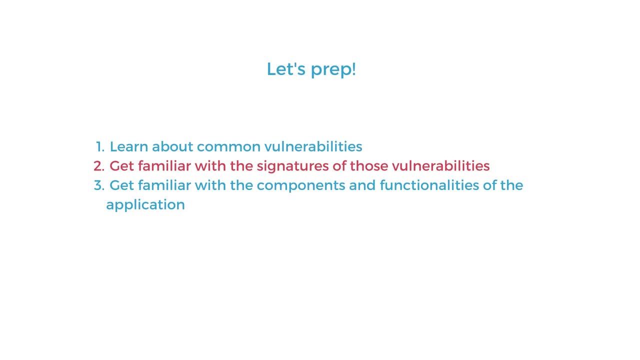 for instance. So specifically, you should try to arm yourself with the knowledge of what these vulnerabilities look like in your application's context. Although different vulnerability types have common patterns in code, these patterns can look quite different- experiência Learning- what common vulnerabilities look like in the context you're working with. 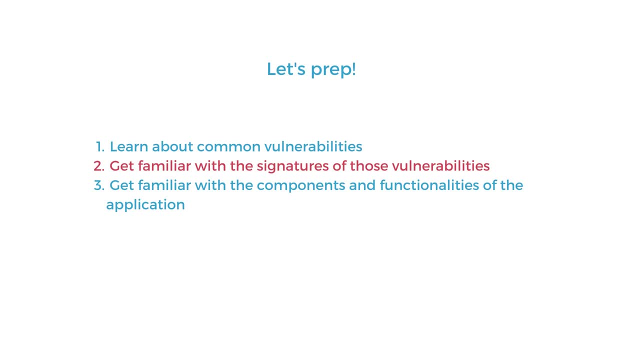 will help you spot patterns more accurately and faster. Next up, if you did not build the application yourself, try to get familiar with the functionalities and the components of the application. Let's say that you learned a certain typo to create a pattern in your website. 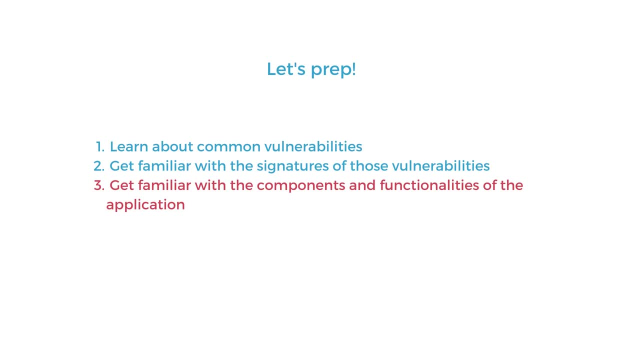 Or you can use muscle files tokiem there, So that way you can create competition from opportunities and podcasts out, for instance, who its users are, what each user can do, what kind of data is the application processing and what are the business impacts of each feature. This will help you. 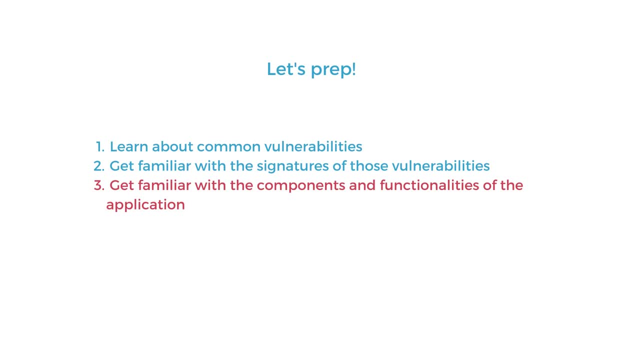 prioritize your analysis down the line, because if you cannot audit the entire code base manually, then you should start with the parts of the application that poses the highest risk to the application's users and its business. So let's start analyzing some code First. 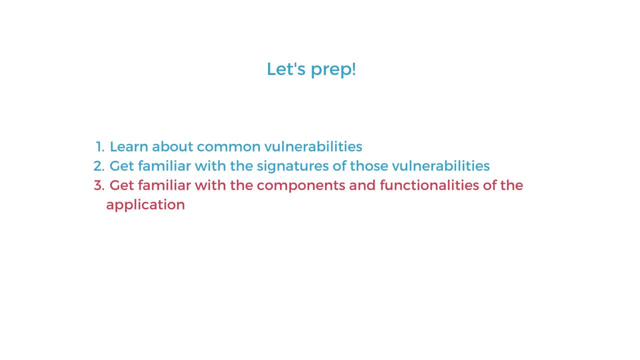 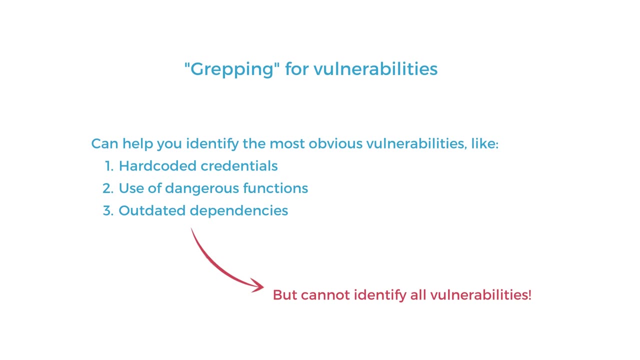 if you are short on time, focus on searching for the most common and the most severe issues. A quick way to do this is by starting to search for strings, keywords or code patterns that are known to be indicators of vulnerabilities or misconfigurations, For instance hard-coded. 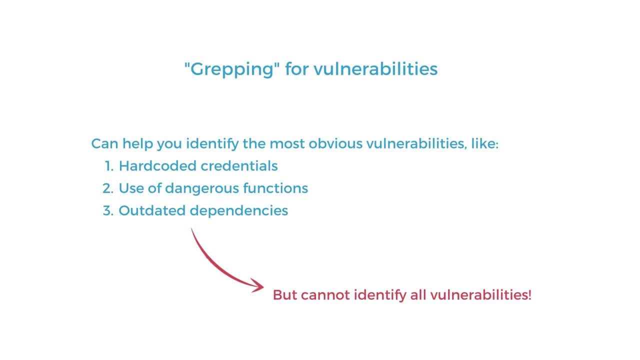 credentials like API keys, encryption keys and so on. If you are short on time, then you should, and database passwords can be discovered by searching for keywords in the code base, like key, secret password or a regex search for hex strings or base64 strings. 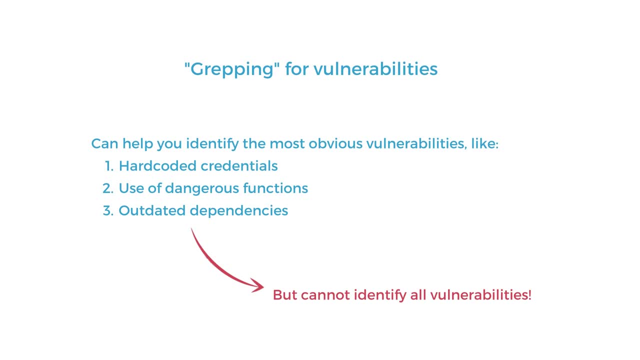 Another vulnerability that you can look for is the unchecked use of dangerous functions. Search for the code base for the use of dangerous functions and see if any of them are reachable by user-controlled data. For example, you can search for strings like system or eval. 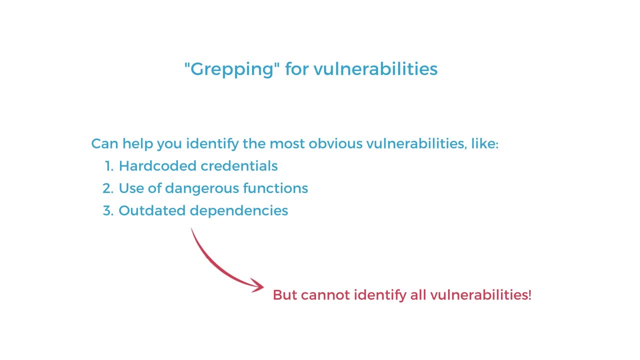 for potential command injections. And then you can also browse through your dependencies to see if any of them are outdated. And remember that I talked about getting familiar with the functionalities and the components of an application right After searching for these obvious issues like hard-coded secrets, the use of dangerous functions and the use of outdated 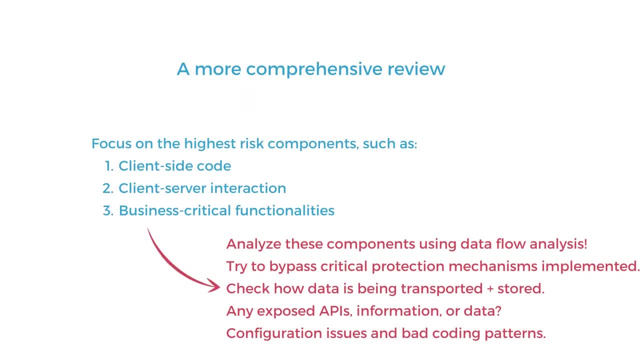 dependencies. start analyzing in detail. Also, make sure that you have everything you need to do your best to solve the application that will pose the highest risk to its users and its business. These are usually places where the client interacts with the server, because these are the places where malicious input can enter the 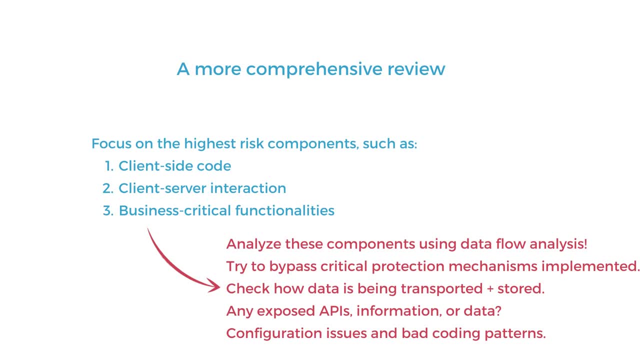 application. So first examine your client-side code for security flaws. Your client-side code is something that you should pay attention to, because that's where the users interact with first, And then focus on code that deals with user input, that the application takes in- user input like HTTP request parameters, database queries, file reads. 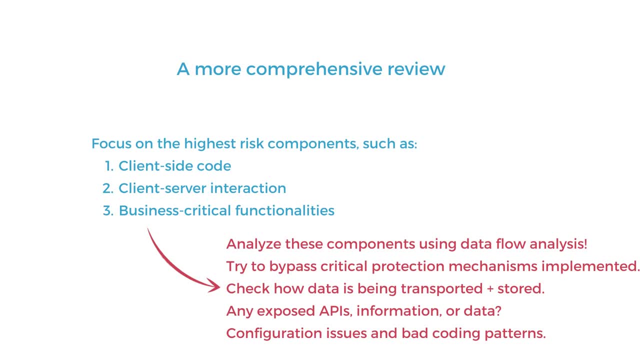 and file uploads. these functionalities provide the entry points for attackers to exploit the application's vulnerabilities. Trace the data flow of user input from these functionalities to other functions and see if they can reach dangerous sync functions. Tracing data flow like this to corresponding syncs can help you identify many, many common vulnerabilities, like cross-site. 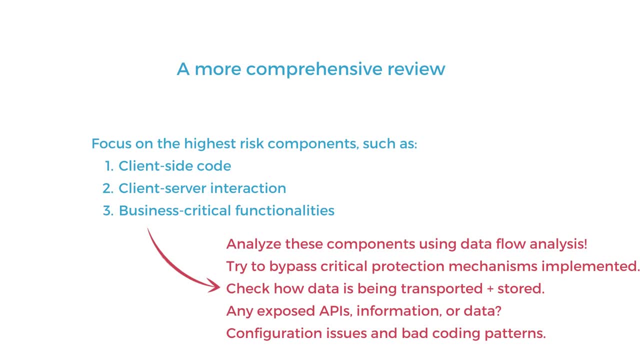 scripting, SQL injections and shell uploads, And then review the code that performs critical functionalities in the application. This includes code that deals with authorization, authentication, functionalities that deal with sensitive data and other logic that is critical to your business functionality. So look at the protection mechanisms implemented in these functionalities and see if you can bypass. 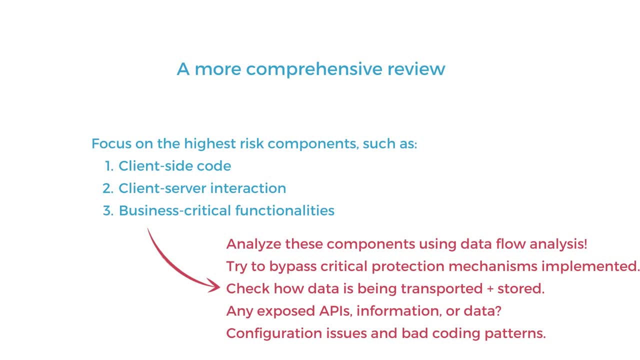 them And, at the same time, check how these functionalities are dealing with sensitive information. Check how business data and user data is being transported. Are they being transported and stored in a safe way? This is also a good time to look for exposed APIs. Look at the endpoints that you have available.